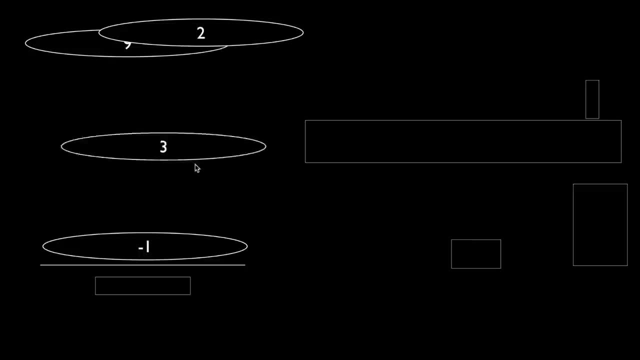 So you could have minus one at the bottom, And then you can put three, And then let's say this one, nine, this pancake right here, And then at the top you can put this one, And then you might say: okay, what if I want to retrieve this pancake right here with the number three written on it. 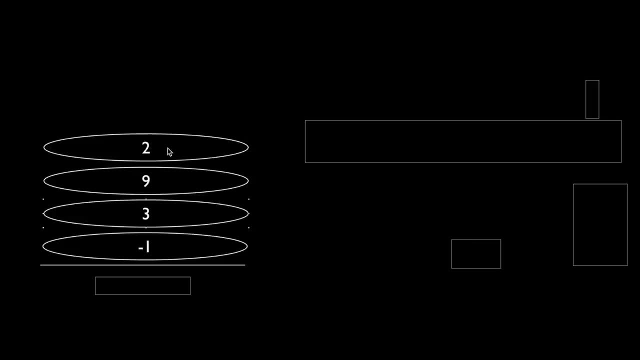 Then what you would need to do is you would need to take out this one first at the top, And then this next one, the nine pancake, And then, finally, you can take out this one first at the top. So that's how you know pancakes in the real world work. 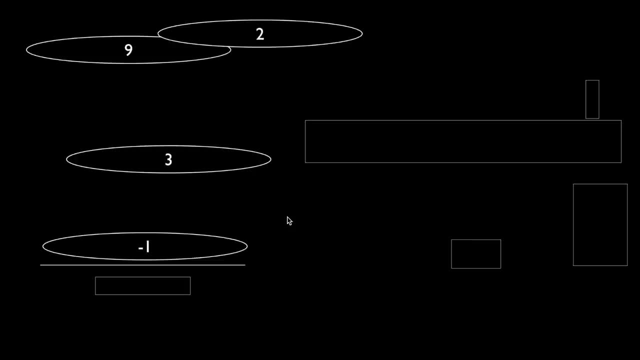 And it's the same thing with the stack data structure. So a stack is a collection of data in which you can only add a piece of data at the top of this structure or retrieve a piece of data from the top of this structure, So you aren't really able to retrieve data from any position. 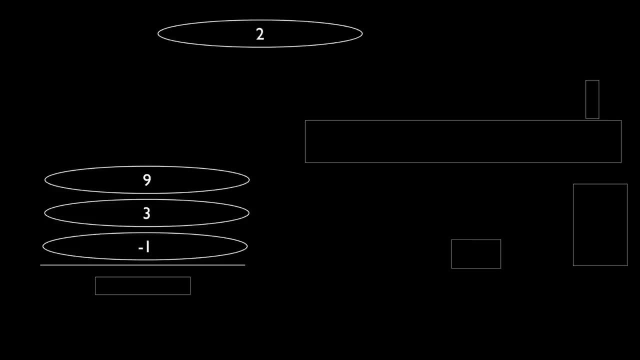 Just like this, Just like you could, for example, in an array. So another way to describe the same thing is that whatever piece of data you put in last will need to come out first. So in the current structure of these three pieces of data, the last piece of data that we put in is nine. 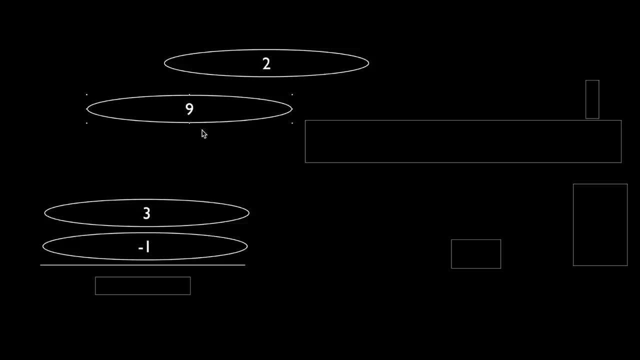 So that needs to come out first, And that's sometimes referred to as last in, first out. Okay, so that's how a stack works, But how can we implement it? Well, one way to implement it is by using an array. 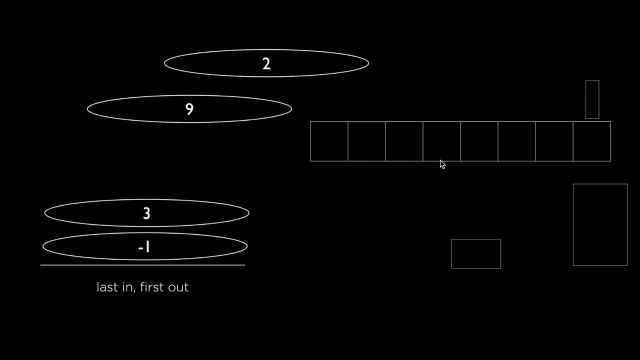 So we have an array of eight elements here And we're going to try to represent this stack right here. To do that, the first thing we'll need to do is we'll need to have a pointer or just an integer variable. that's going to point to the last element that we put in. 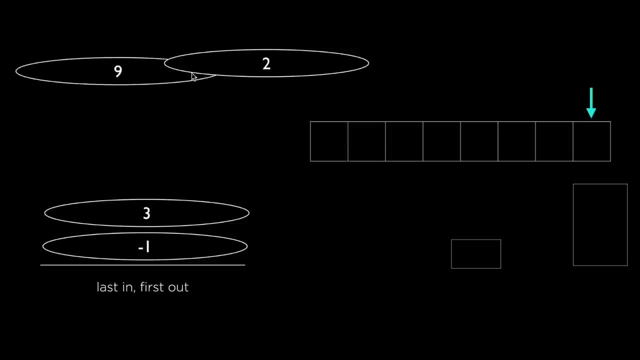 In this data structure And let's say for now that the stack is empty, Then there's no last element to point to, so we can initialize this variable to minus one or the index that would be here, but that doesn't exist, And this shows that this stack is empty. 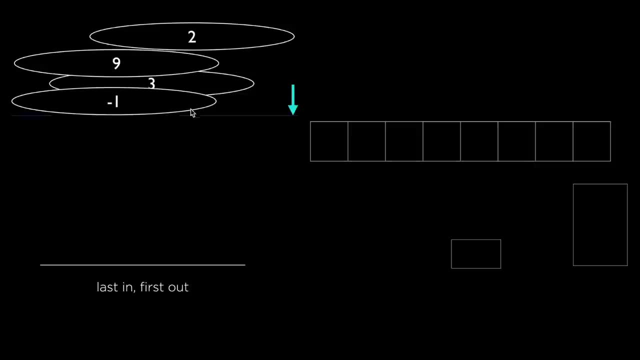 And now what? if we want to start putting in some piece of data here, For example, minus one here, then what we can do is move the pointer here Again. this is going to always point to the last element that we put in in this data structure. 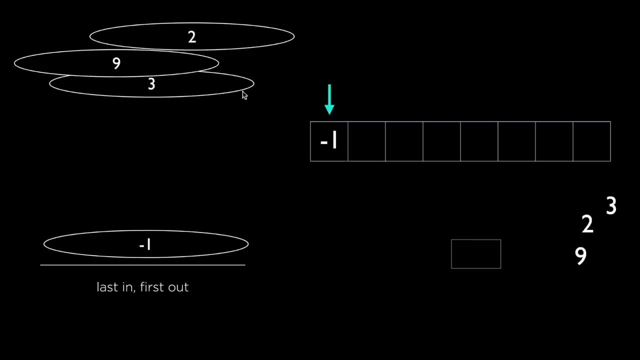 And then put minus one here. And what if we want to put in three on top of minus one? then we can move the pointer again, again pointing to the last element that we put in, and then put three here, and then we can keep doing that. 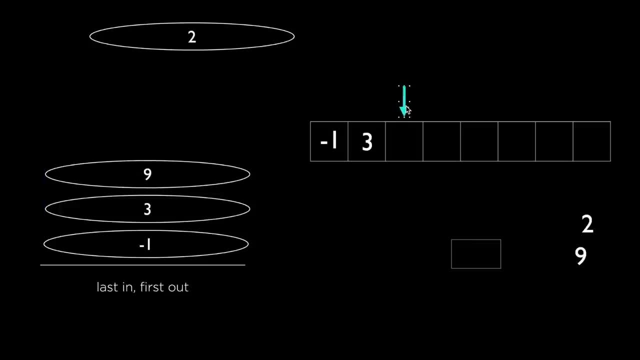 If we want to put nine here, you can move the pointer here or increment pointer by one And then put nine here. And what if you want to remove this number right here, nine? To do that, all you need to do is you need to move the pointer back by one or decrement this variable by one. 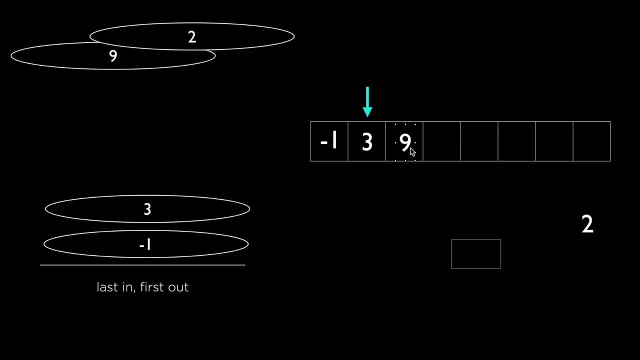 Now you could do something with this number right here. You know either erase it or change it to something else. You know either erase it or change it to something else else, but it doesn't really matter, because in this data structure we always know that the pointer. 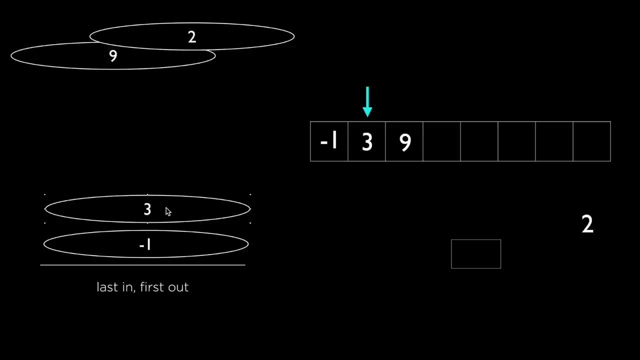 always points to the number that's at the top of this structure, so the numbers following this pointer are not relevant. so we can keep going like this. if you want to put in 2 here, you can move the pointer back here and then update this number right here with 2. 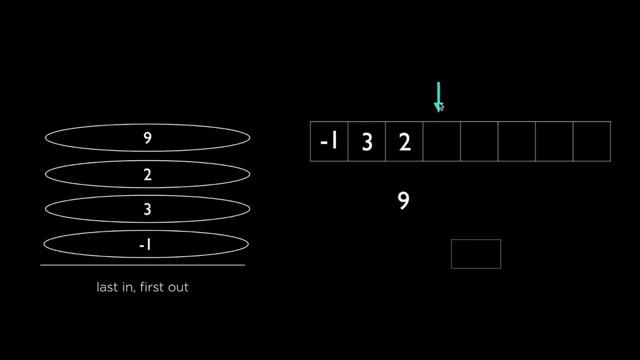 and then, if you want to put 9 again here, you can move the pointer by 1 and then put 9 here and throughout this explanation we saw a few key operations here. one is delete. sometimes it's called pop, that's deleting or removing a number. 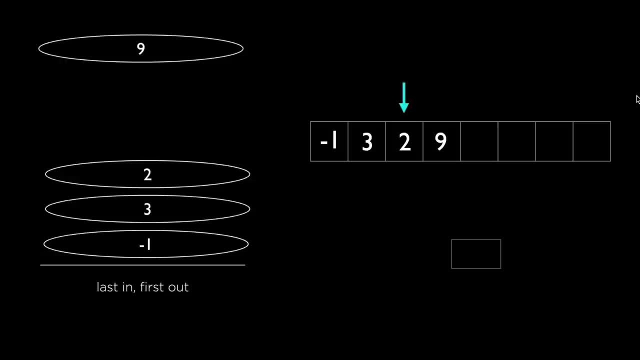 from this data structure, and another one is add, and that's adding a number on top of this data structure, and with this particular implementation, you can implement both of them in all of one or in a constant amount of time, and that's assuming that the number of elements that we put in 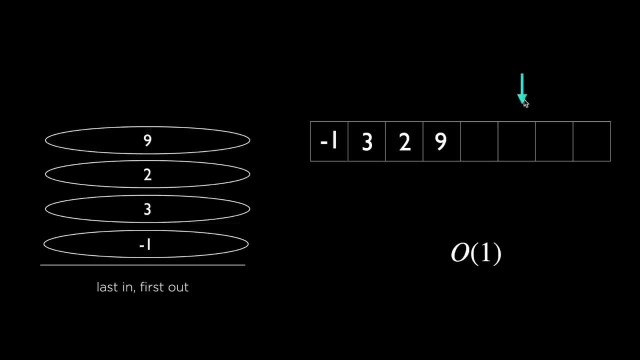 in this data structure doesn't exceed the length of the array, and if it does, you would need to either zero an element or limit all the distance error, or make a new array that's longer than the original array and transfer all the elements from the first array to the second array, and that would take some. 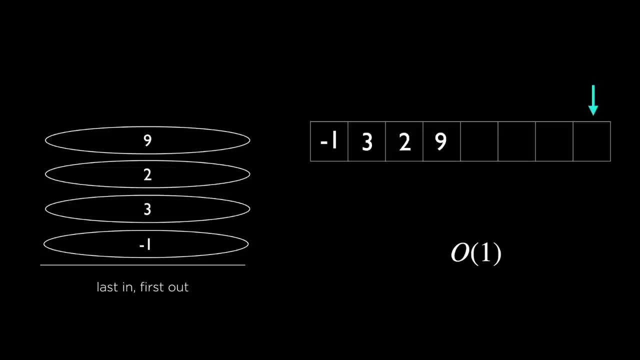 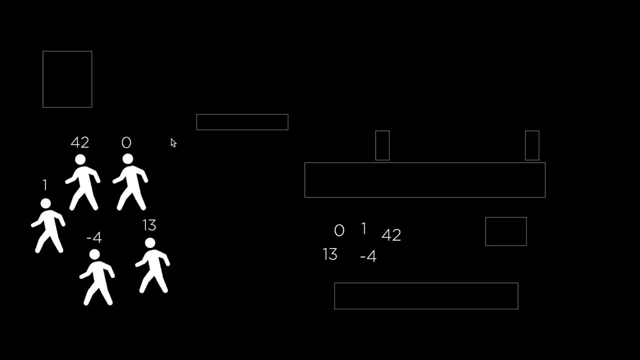 extra time. anyway, that's it for a stack. let's now take a look at a queue. the analogy I use to understand a queue is a bunch of people lining up in a line or in a queue. so let's say we have these people with some numbers assigned to. 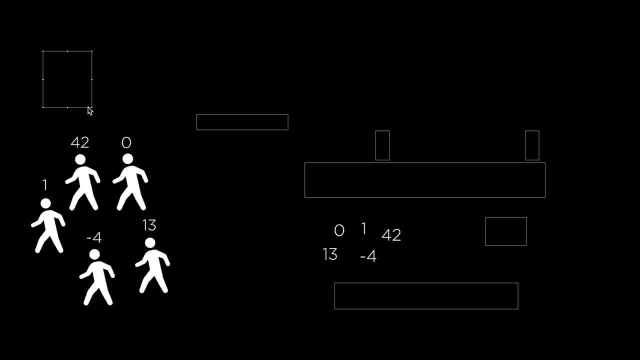 them just for convenience and they want to line up to do something, for example to see this octopus, for whatever reason, and this octopus is busy, so they need to line up and with a cue, I think you already know how it works, but you can put people in the queue or in this line and when the octopus is free, the person 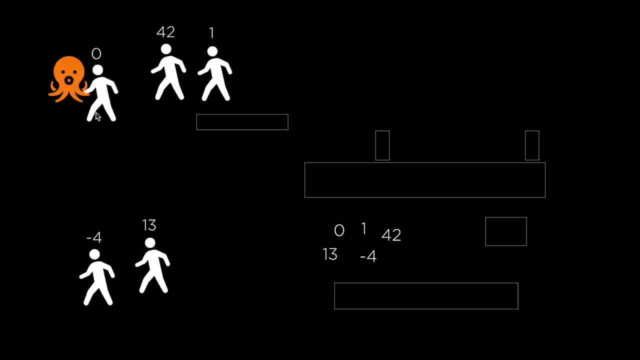 that's at the front of the queue. knowledge is being covered on this line. the queue can see the octopus and then go away, and then you can add more people in the queue or more numbers in the queue, and then the person or the number that's in front of the queue. 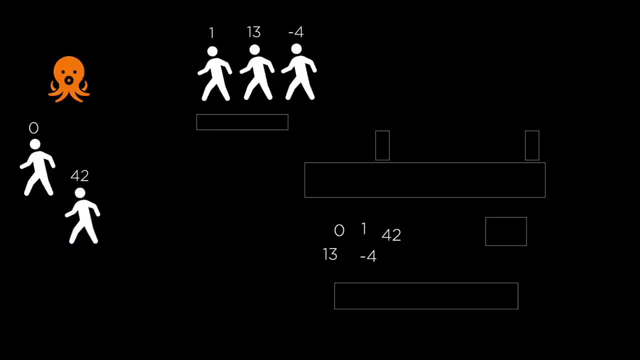 can see the octopus and then go away. so that's the idea of the queue data structure and i think you can see that whatever number or whatever person that came in first will go out first. two out of this data structure and that's sometimes referred as first in, first out. 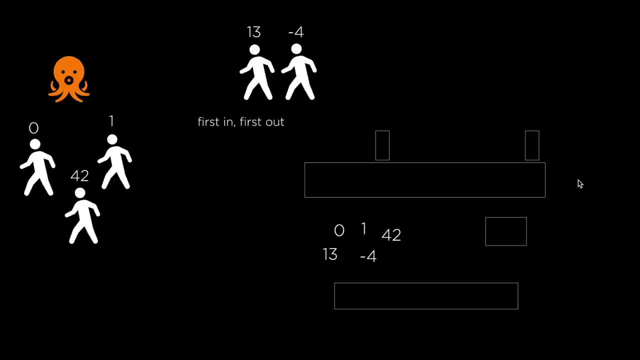 okay, and how can we implement this data structure? one way to implement it is with an array again, and this time we're going to have two pointers. the first one is going to point to whatever is at the front of the queue or, in this particular example, this number or this person right here, and we're going to put 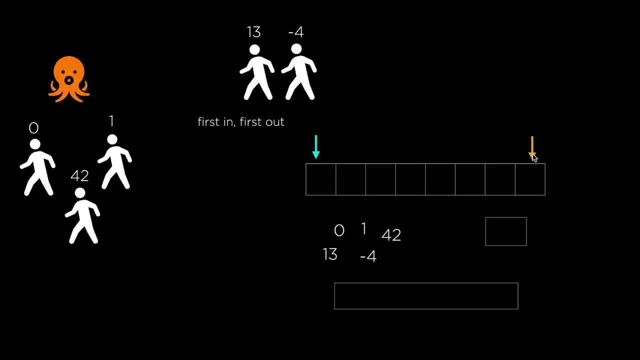 this one right here, at zero, for now. and the second pointer is going to point to the space that's right after the last person or the last number in the queue, and for now i'm going to put this at the same position as the first pointer, at zero, and let's say that the queue is empty right now. 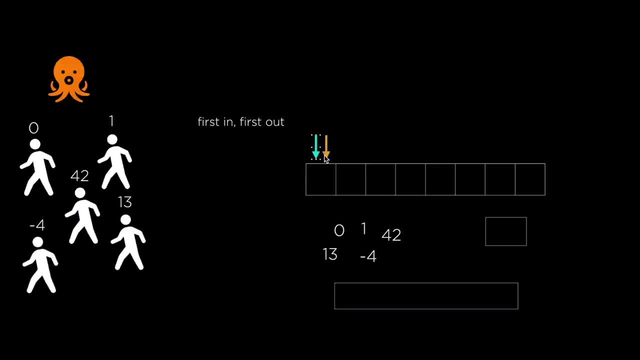 then we're going to make these pointers be initialized to both zero right here, and we're going to implement this data structure so that, whenever these two pointers point at the same thing, this queue is empty. okay, now let's think about how we can represent a line of people with this. 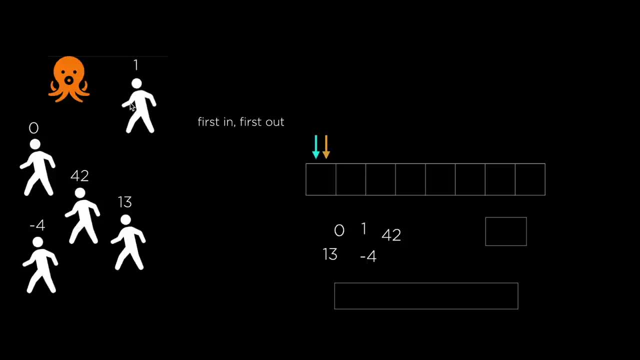 particular implementation. so let's say that this person comes in the line of people and we're going to put this at the same position as the last person, and if we're at the same line first, then we can put number one here and then move the second pointer. 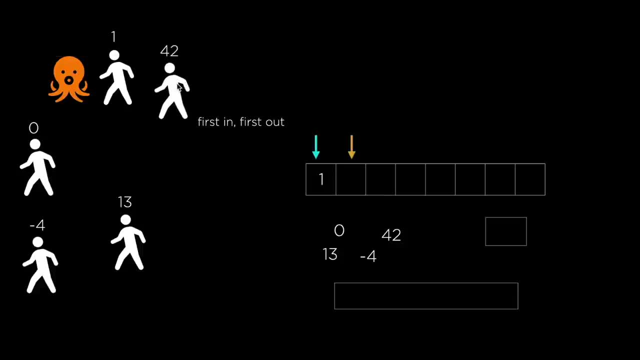 right here, and if there's another person right after that- let's say 42- then we can put 42 here and then move the pointer here again. the first pointer will always be pointing at the first person in the queue or the front of the queue, and the second pointer will always be pointing at the front67. 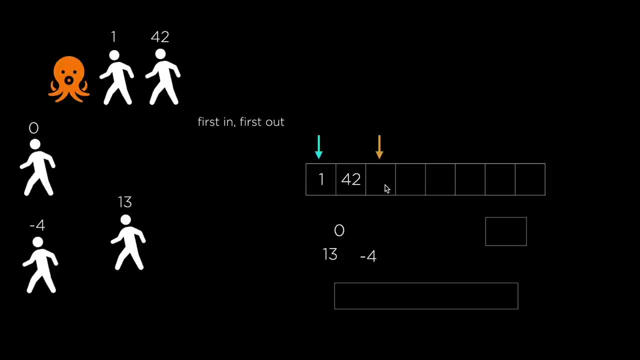 the second pointer will always be pointing at the front57, be pointing at the space right after the last person or the last number in the queue. so let's keep going with this. if 13 comes in a line, we can put 13 here and then move the pointer. move the second pointer right here. and what if? 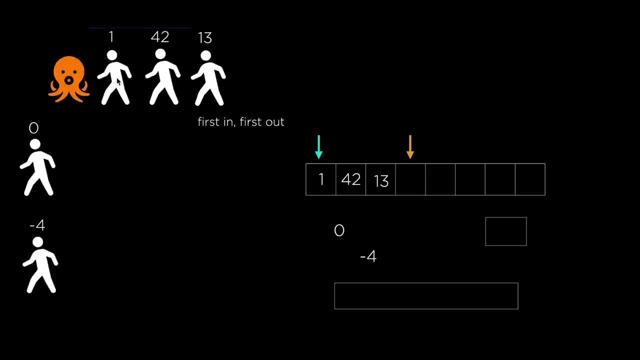 the octopus is free now and this person 1- sees the octopus and goes away, then we can just move the first pointer over here and we don't really have to do anything with this number right here. 1, because in this implementation we'll know that the queue is only between these two pointers, so we can just keep. 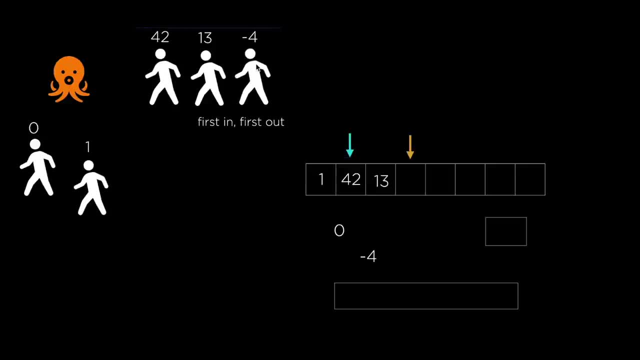 going like that and just to show you more examples: if minus 4 comes after that, we can put minus 4 here and then move the second pointer over here. if 0 comes after that, we can put 0 here and move the second pointer over here or increment the second. 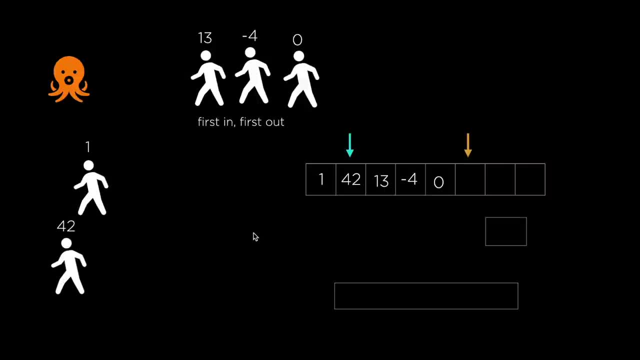 pointer by 1.. And if 42 goes away, we can move the first pointer over here. Let me just keep going like this. And what if you have a situation like this now, where you have three people in the queue- 0,, 1, and 42, and you want to add another person- minus 4- here. To do that, we can put minus 4 here. 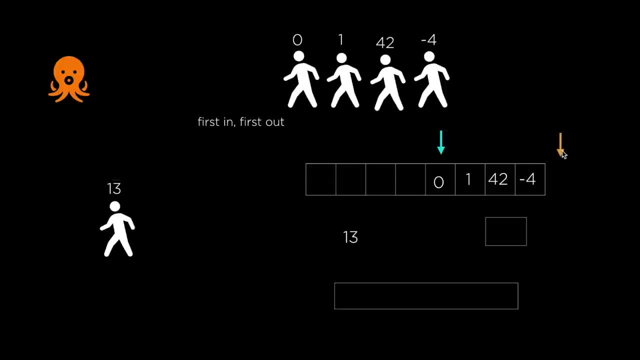 and then you would try to move the second pointer over here, but that's out of bound. To fix that, you can just move this pointer back here at 0 instead. So you can actually visualize this array like a circular array where if you try to go out of bound, you just go back to 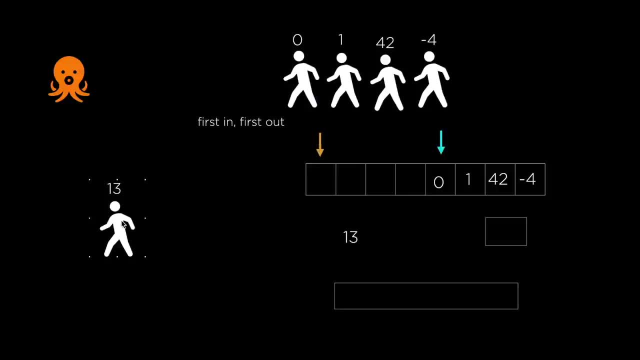 0. So let's just keep going like that. If you want to put 13 after that, you can put 13 here and then move the second pointer by 1 over here, And it would work the same way for the first pointer too. 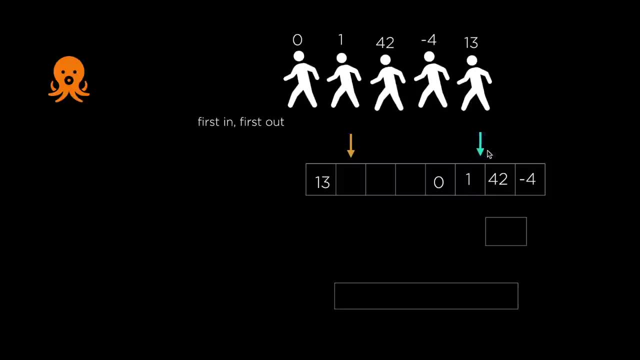 If the first pointer keeps going to the right and if it's about to go out of bound, instead of having it go out of bound, we can just bring it back to 0, right here. And another thing to note about this particular implementation is that you're only able to store. 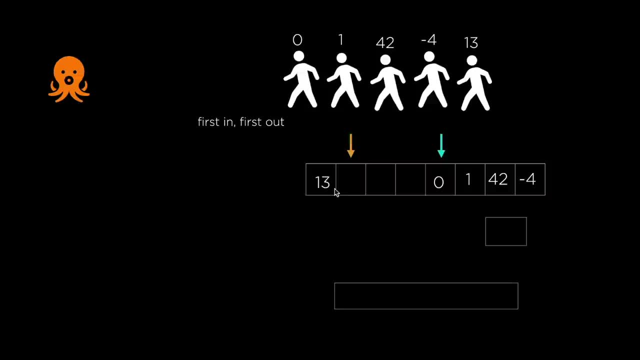 at most n minus 1 elements in this data structure, assuming that the length of the array is n. To explain that, let's consider this situation where we have the second pointer right here and we have some elements here, here and here, If you try to add one more element right here. 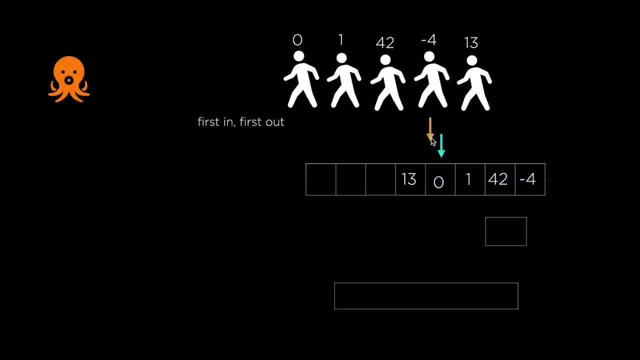 you would need to move the second pointer right here to the same position as the first pointer. But we've already said that in this particular implementation, if these two pointers point to the same thing, this queue is empty. But clearly it's not empty And that's why we would need to. 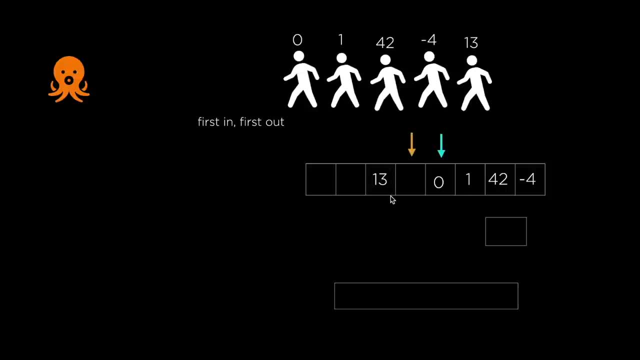 stop here, And that's why we're only able to store n minus 1 elements where the length of the array is n. If you want to store more elements, you would need to either throw an error or create a new array that's longer than the original array. 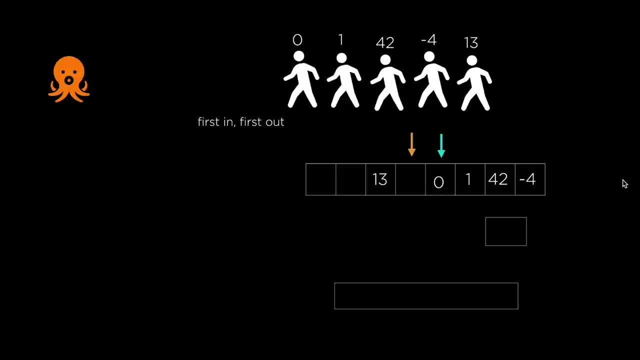 and then transfer all the elements to the new array. Anyway, in this implementation we saw two key operations. One is removing an element or a person or a piece of data from the queue, And another one is adding a piece of data to the queue. Sometimes, 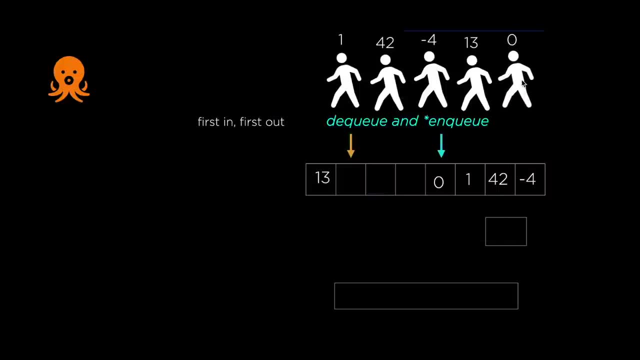 it's called dequeue and queue And with this particular implementation, assuming that the number of elements doesn't exceed n minus one, we can implement both of those things in O or in constant time. And that's it for a queue. But let's quickly discuss another data structure. 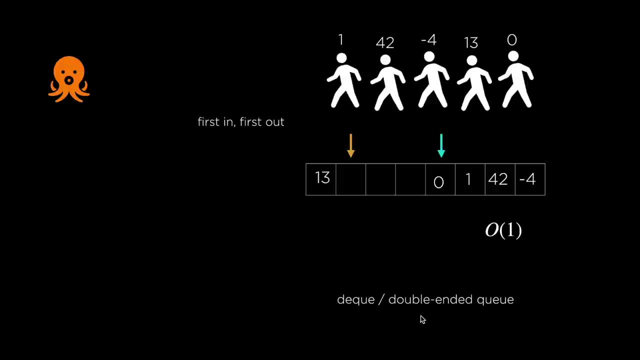 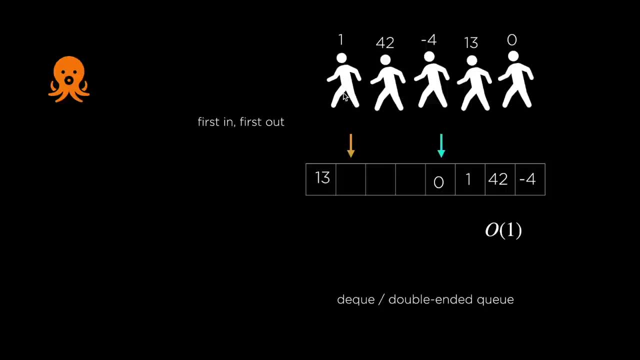 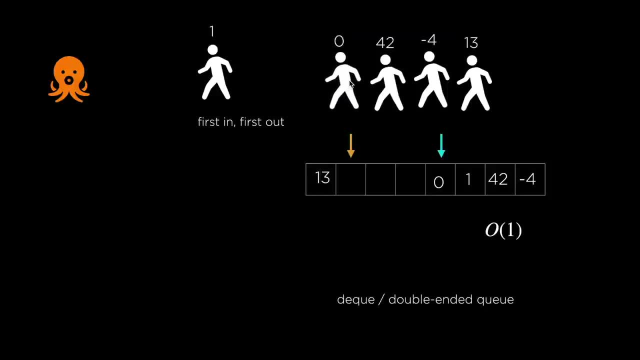 right here and you can add a person at the front of the queue or at the left side of the queue, or add this piece of data at the right side of the queue, and one way to implement this is similar to the implementation of the queue that we. 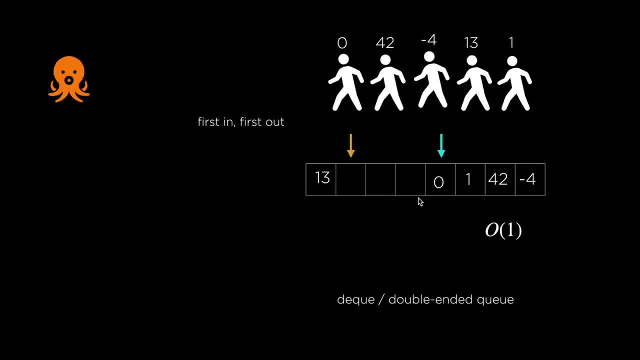 saw. so you can use a circular array still and have the same kind of structure, but in this new structure we're able to remove data from either end and add data to either end too, so you would basically have functions that are called something like add left, remove left, add right and remove right sometimes. 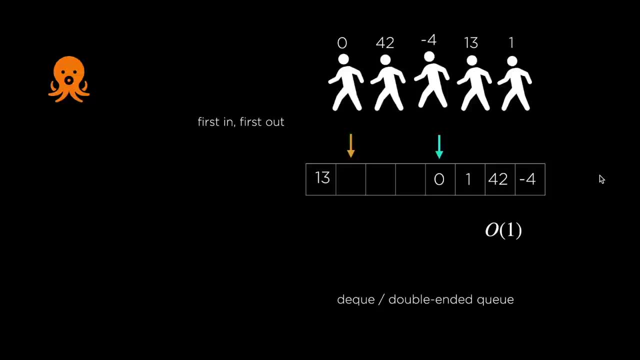 they're called pop left, pop right or other names, but these objects are in both of these cases. so you can see that here in the other names. so you could see that here in the other names. so you could see that here in the other names. so you could see that here in the. 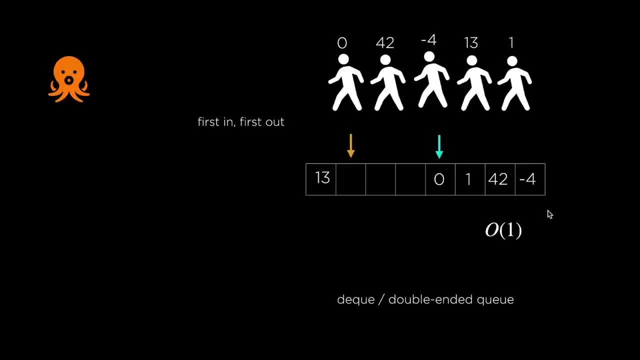 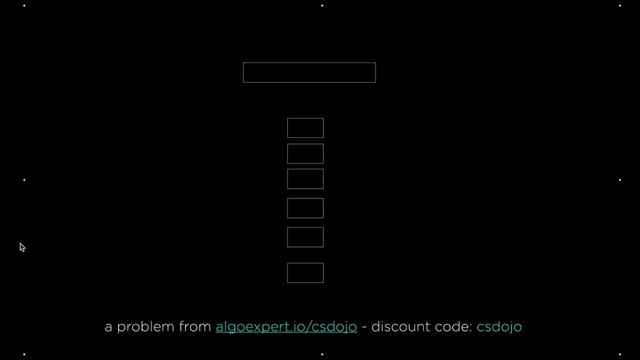 you get the idea you should be able to implement all of those operations in o of one as well. okay, so that's my introduction to these three data structures, but if you want to practice using these concepts, one of the resources i recommend is one of my business affiliates, algorexpertio.